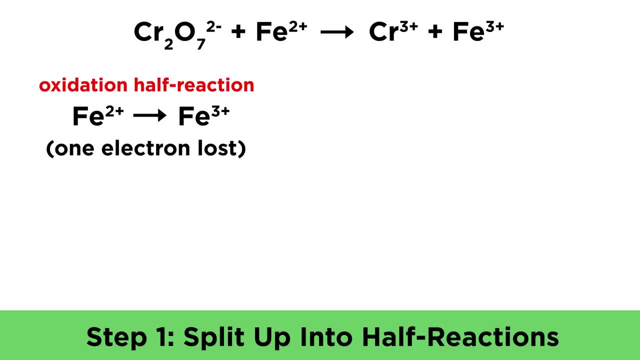 This is the oxidation half reaction because the iron has lost another electron For the reduction half reaction. iron 2 plus becomes iron 3 plus. This is the oxidation half reaction because the iron has lost another electron For the reduction half reaction. dichromate becomes chromium 3.. 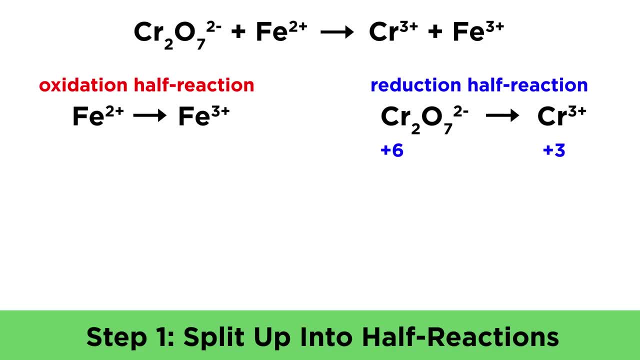 We can see by looking at the oxidation numbers for chromium that it has been reduced. Now we must balance each half reaction starting with elements other than hydrogen or oxygen. We can see that for the reduction we need to put a two here to get two chromium atoms. 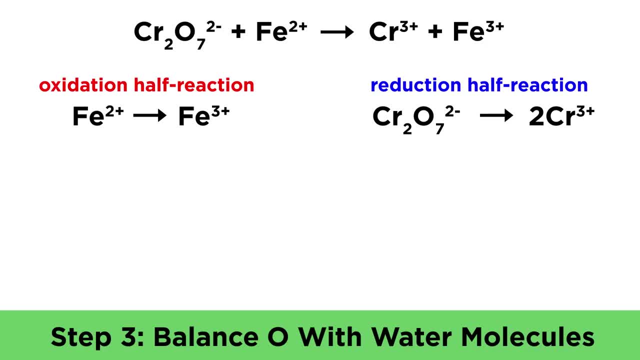 on each side. Next, we balance oxygen by adding water molecules. We have seven oxygen atoms on the left, So we need to add seven water molecules to the right, since there is one oxygen per molecule. Now we can balance hydrogen atoms by adding hydrogen ions. 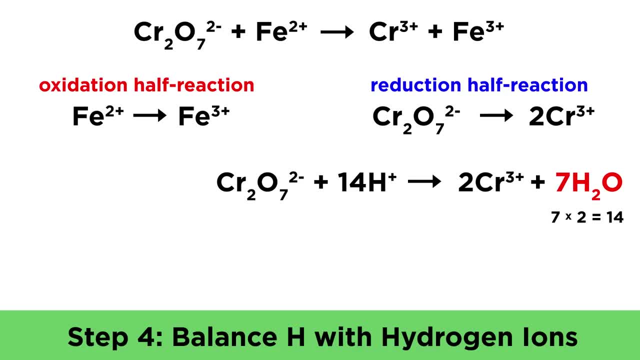 Since there are fourteen hydrogen atoms on the right from the seven water molecules, we will need fourteen hydrogen ions on the left. This means all of the elements are balanced. Now we can balance the electrical charge for each half reaction by adding electrons In the oxidation. in order for iron 2 plus to become iron 3 plus, it must lose an electron. 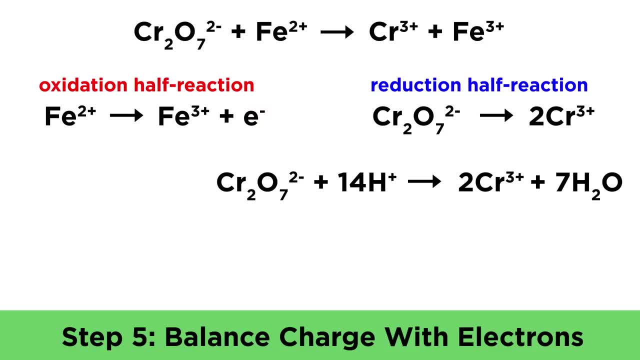 So there must be one electron as a product here For the reduction. it's a little trickier. We have two minus on the dichromate and fourteen H pluses, for a total of 12 plus on the left. On the right we have two chromium 3 ions, for a total of 6 plus. 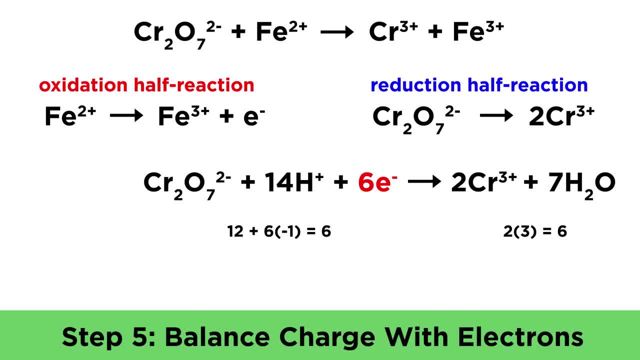 In order to balance this, we will need six electrons on the left to bring the charge down to 6 plus and balance the charge. Now we will need to combine these into a chromium 3 ion In such a way so as to cancel out the electrons. 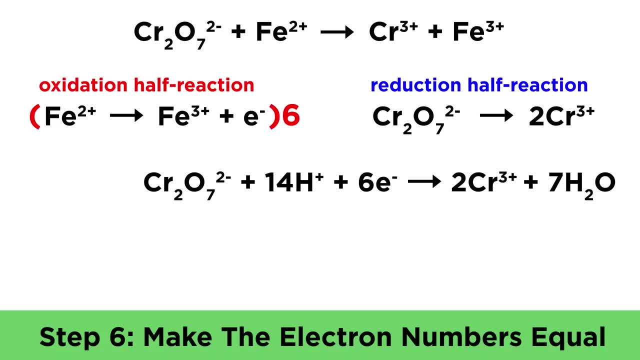 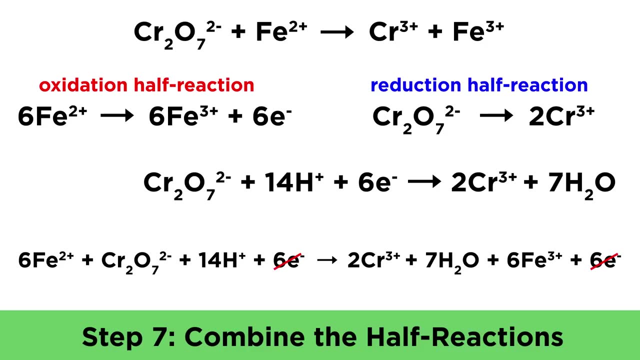 That means we will have to multiply this half reaction by six in order to get six electrons to match the other half reaction. So six of each iron ion and the six electrons we need. Now we can finally combine these half reactions. Once they are combined, we can cancel out any species that appear on both sides which 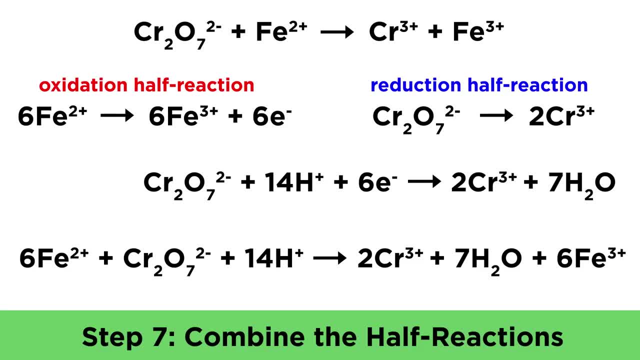 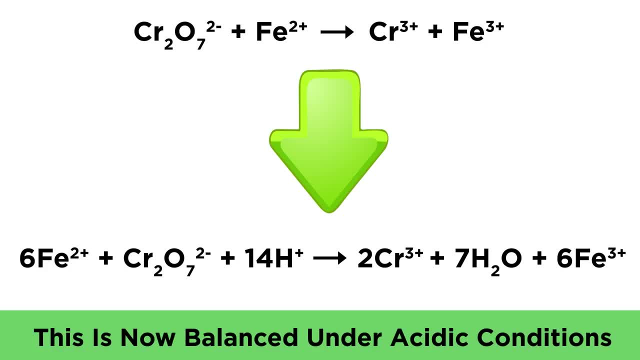 in this case, is just the electrons, So we can now see the exact number of ions that must react In order to produce this particular redox reaction. Let's make sure to realize that this is the algorithm we can use under acidic conditions, which is why hydrogen ions are present. 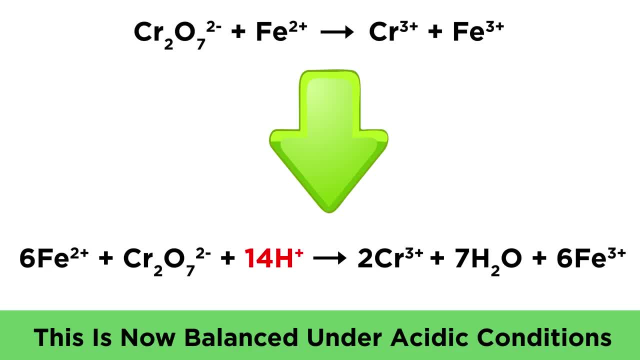 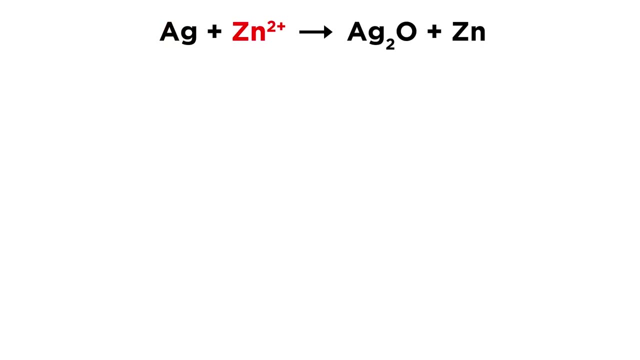 If this is occurring under basic conditions, the algorithm will be just a little bit different, but it will start out by balancing as though we are under acidic conditions. So let's do that first, just as we have learned. Let's say we have some solid silver reacting with zinc two plus to become silver oxide. 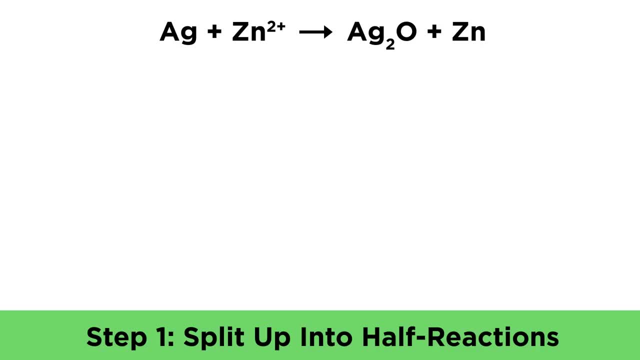 and we want to balance it Again. we will start by separating this into half reactions: Silver has been oxidized, going from zero to plus one, and zinc has been reduced, going from plus two to zero. Then, just as before, we balance elements other than hydrogen and oxygen. 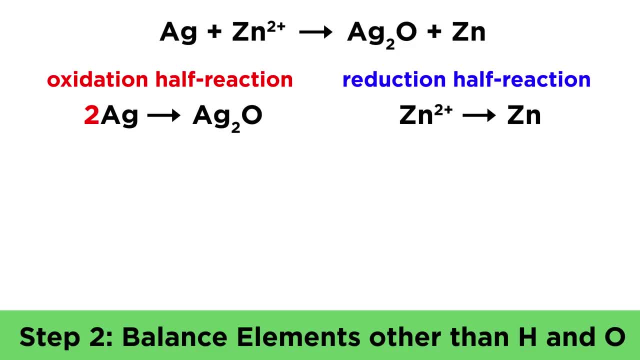 That will involve placing a two here before solid silver. Next we balance oxygen with water molecules. That means one on the left here. Then we balance hydrogens with protons, Which means two on the right here. Then we balance charge by including electrons. 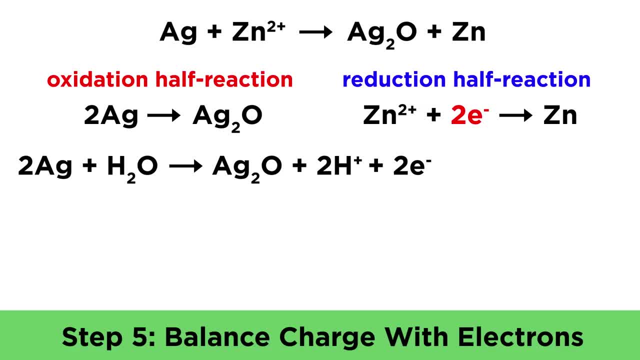 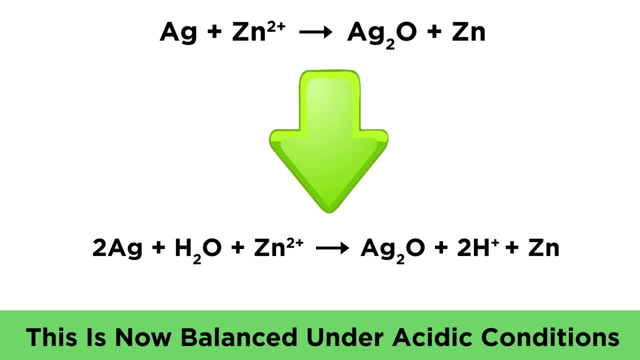 That means two on the right for this one and two on the left for this one. Because the number of electrons in each half reaction is equal, we can go ahead and combine them, cancel out the electrons, and we get this. If conditions were acidic we would be finished, but since they are basic, there is a little. 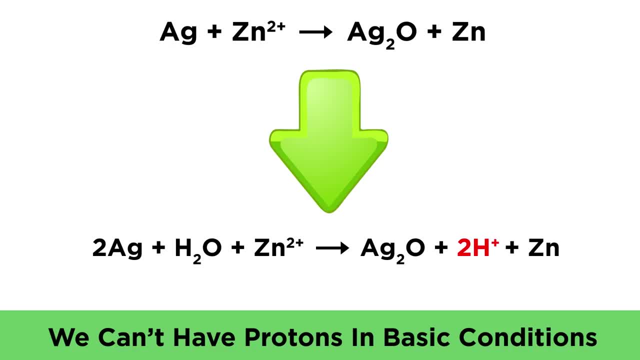 more work to do, because it doesn't make sense to say that protons exist in basic solutions. First we note how many protons there are and we add that number of hydroxides to both sides, So that's two hydroxides on each side. 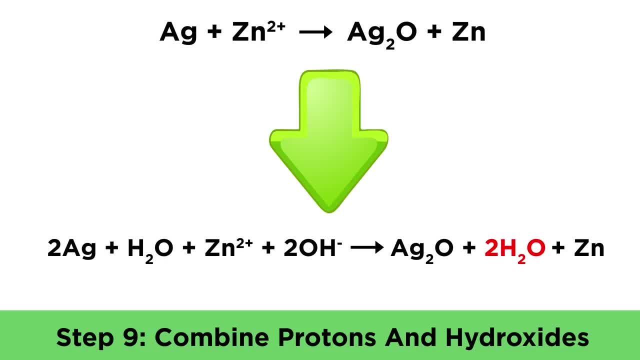 Then, anywhere we see protons and hydroxides, we can combine these to form water molecules, so that makes two waters on the right. Then we cancel any like terms that remain. In this case we can eliminate one water molecule from both sides and this will be the balanced. 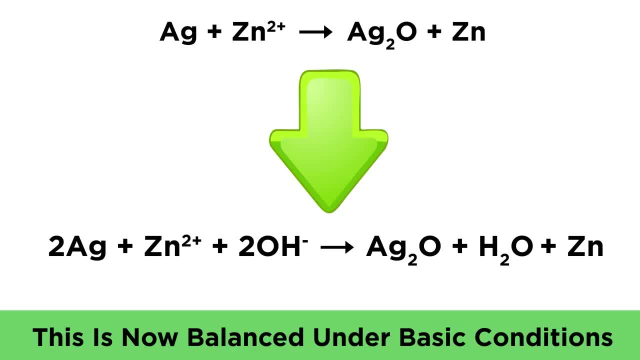 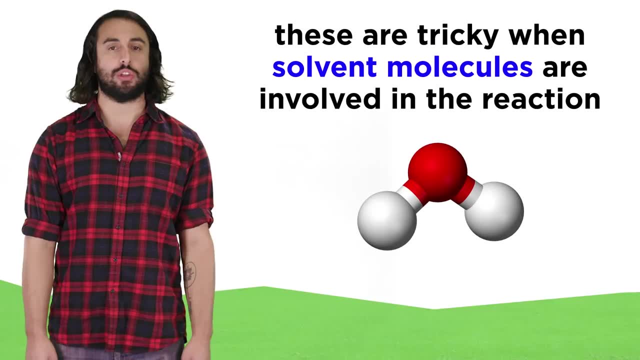 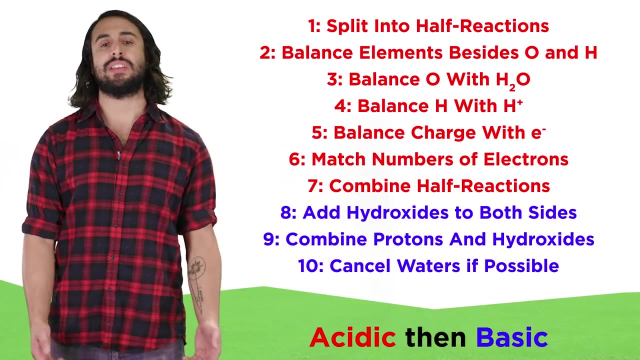 redox reaction under basic solutions. We can see that, in either case, we are involving solvent molecules in order to supply the hydrogens and oxygens necessary for the reaction, and we simply follow a series of steps in order to balance all the components involved.